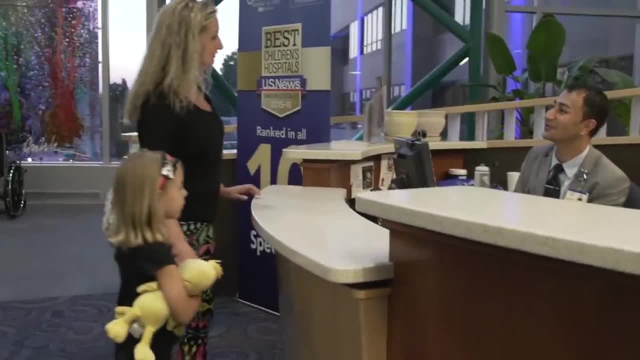 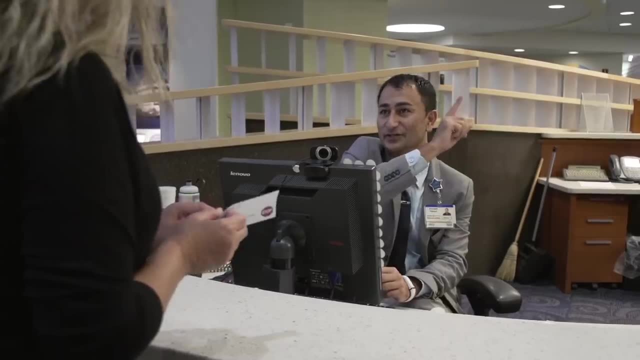 desk to get your name badge to wear during your stay. Good, I need to get a name badge. We're here for a sleep study. Thank you so much. From there, head down to the first floor to get registered for your study. We're here for a sleep study. 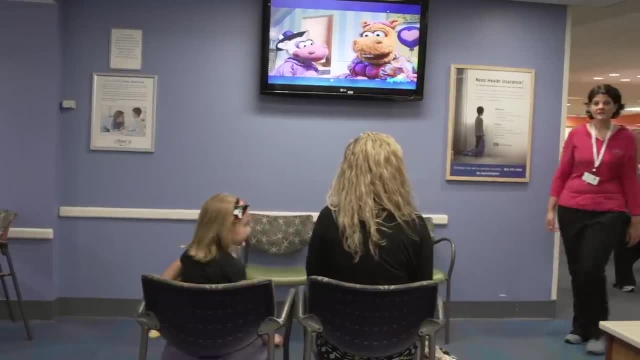 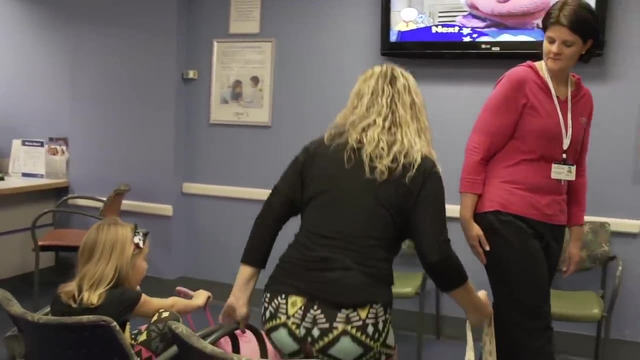 Okay, great, thank you. After a short wait, one of our staff will meet you and walk with you up to the lab. If you want to follow me, I'll take you up to your room. Okay, let's go. Every patient has their own private room with a. 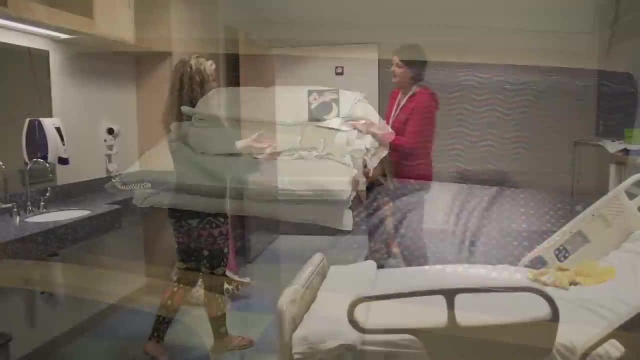 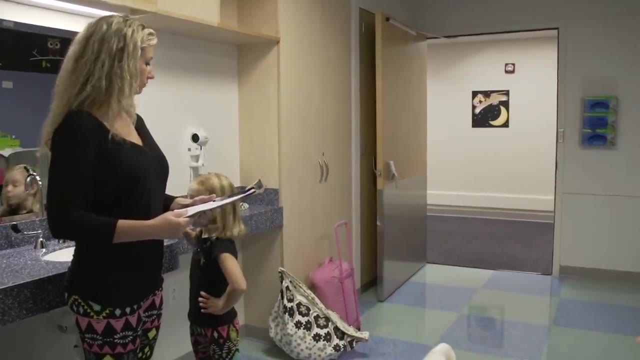 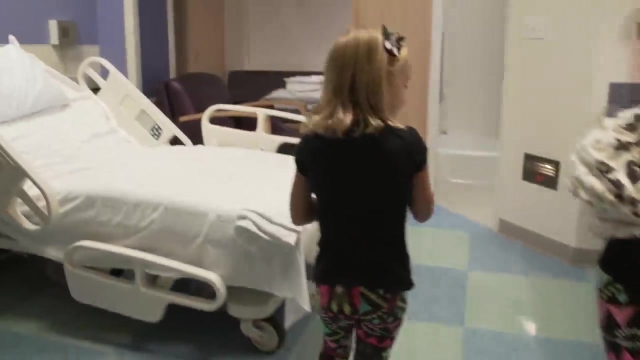 bathroom and pull-out couch to serve as a bed for the parent. Thank you, The technician will have some questions about your recent sleep patterns and will explain what to expect during your stay. At least one parent is required to stay overnight, but siblings should stay at home. You'll have some. 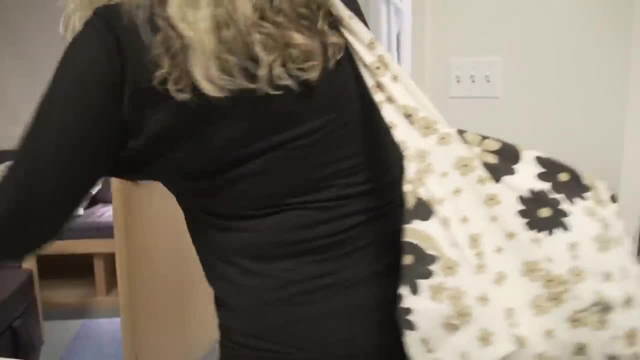 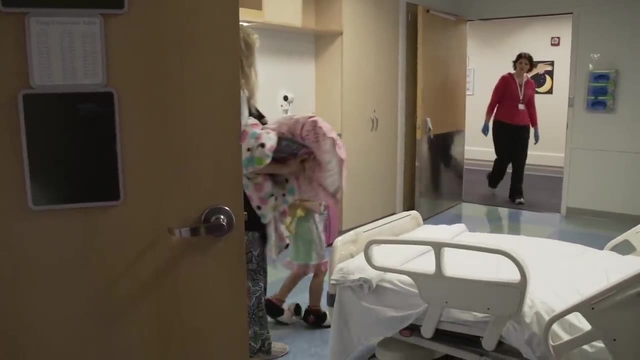 time to change in your pajamas, use the restroom, brush your teeth and do anything else that is a part of your bedtime routine. When the technician returns, it will be time to start the hookup. Okay, guys, you all ready This? 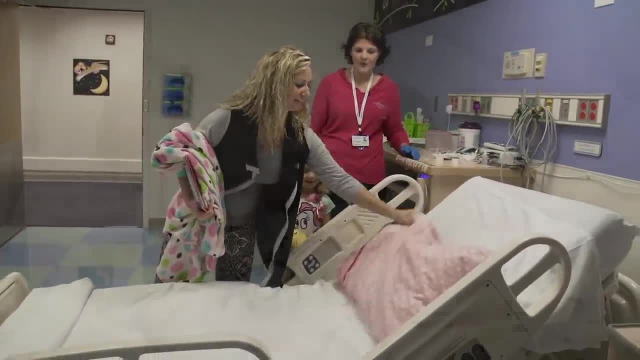 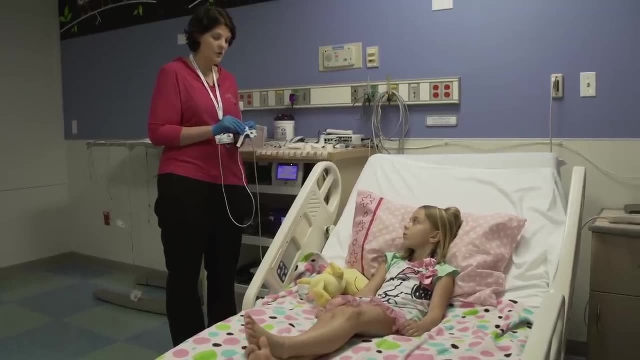 process takes about 40 minutes and is pain free. Okay, Gisela, I'm going to start getting you all set up for your sleep study. The first one I'm going to put on is going to be this cool little nightlight It's. 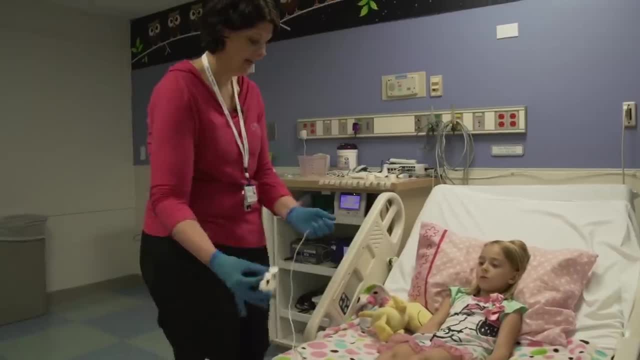 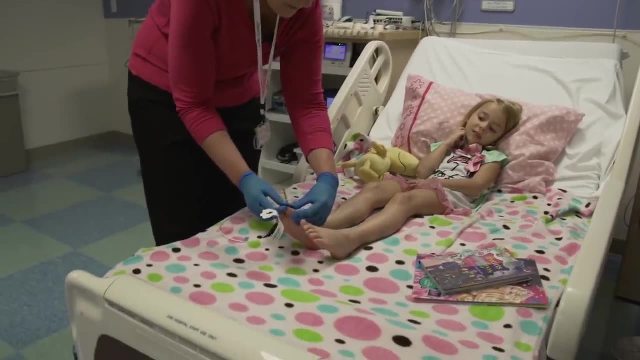 going to go on your toe and it's going to make your toe glow in the dark tonight. Isn't that cool? Yeah, Do you want to touch it? Yeah, Now I'm going to put this on your big toe and put it on with a little piece of. 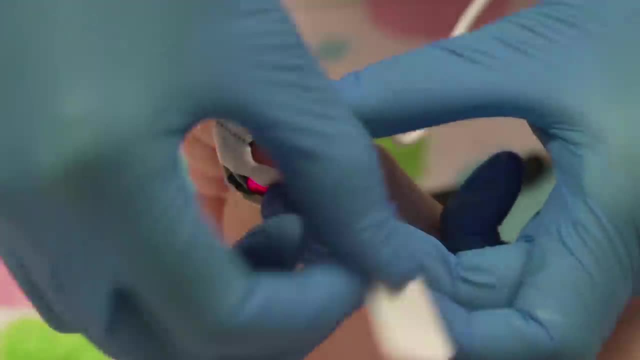 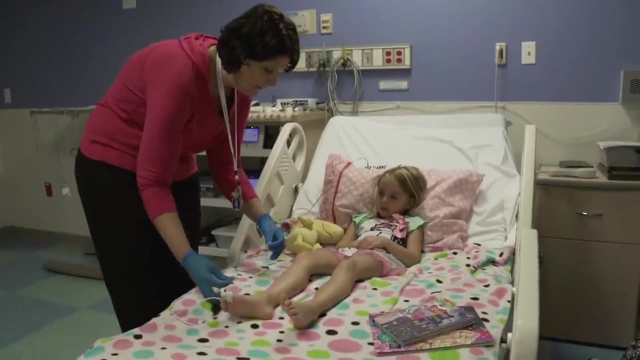 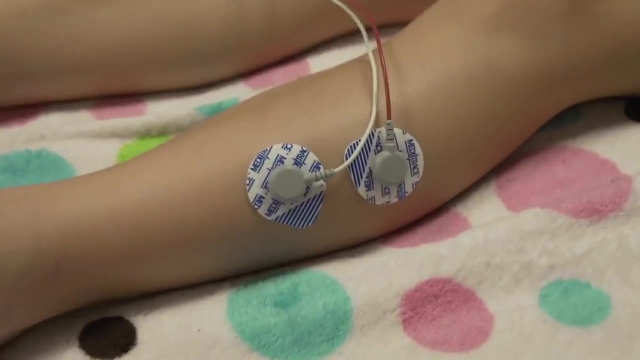 tape: Yeah Done, Yay, Wonderful work. Cold sticker, but it will warm up really fast. okay, You're going to have two stickers on each leg. This is going to go around your chest. It's going to be kind of like a little hug. 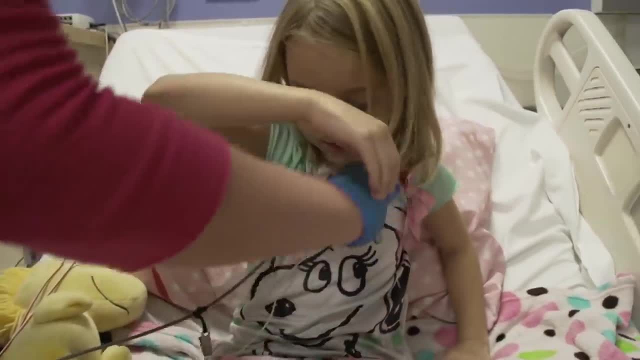 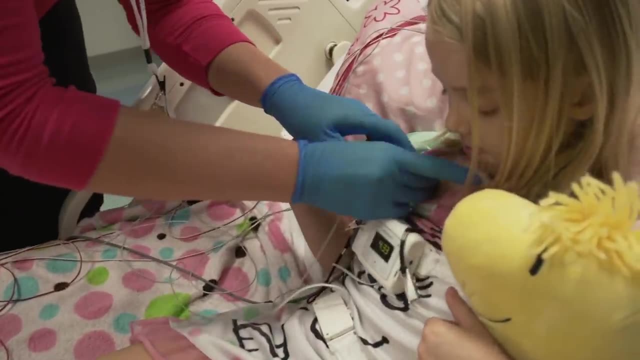 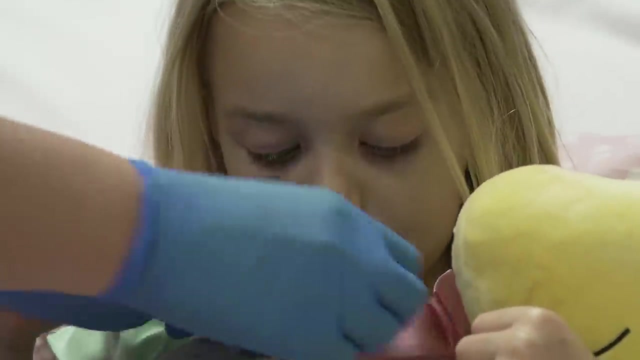 There we go. Next, Gisella, I'm going to put some stickers on your chest. They're going to tell me about your heart tonight. One more sticker for your chest. Okay, Gisella, now I'm going to start putting the stickers and wires that go on your face. 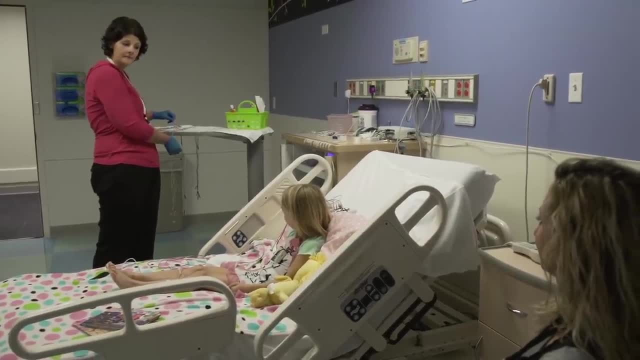 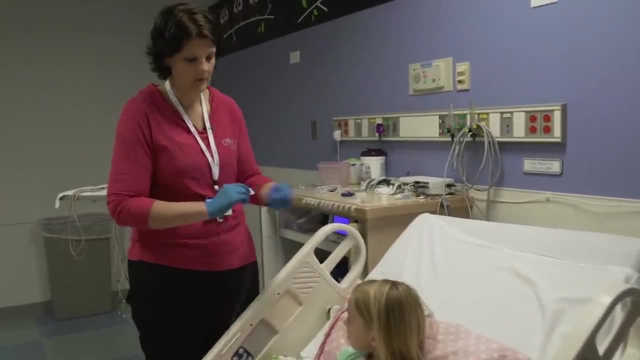 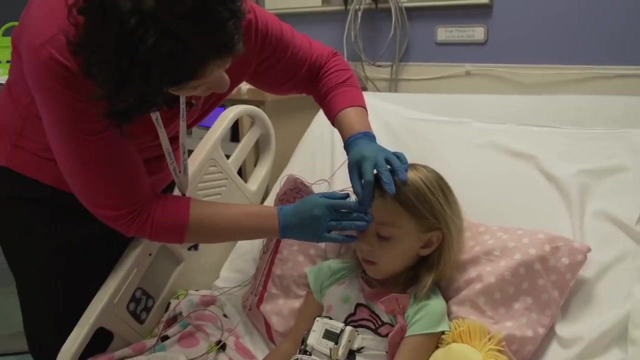 What's your favorite color? Okay? well, the first one I'll put on is pink. So this one's going to go right here on your forehead, right where we cleaned with that special soap. We just smoosh it on there, Just so it sticks. really good tonight. 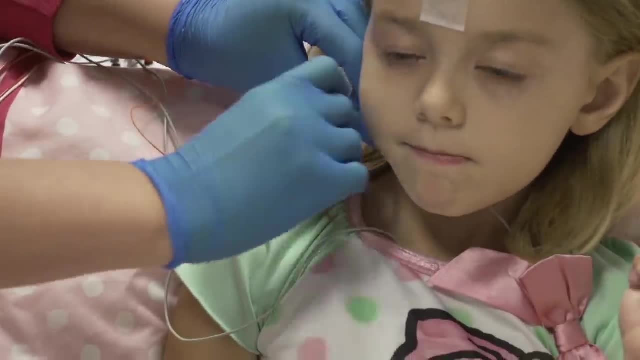 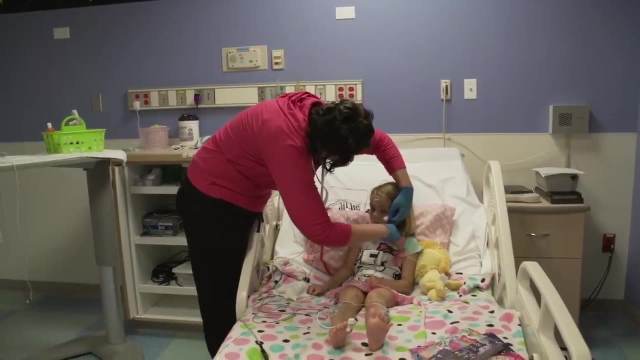 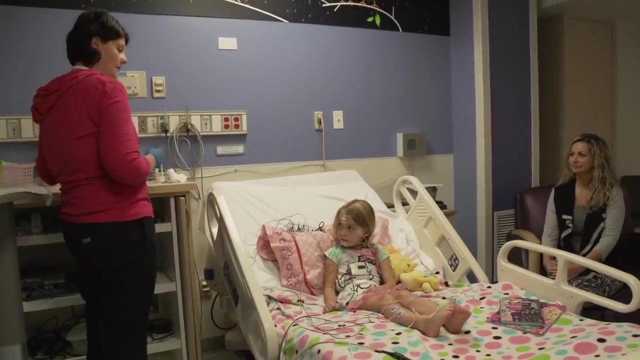 I'm going to put an orange one. This one's going to go down here on your chin. Can you look up like this? Good job, Another one for the other side of your chin. Okay, Gisella, we're all done putting the ones on your face. 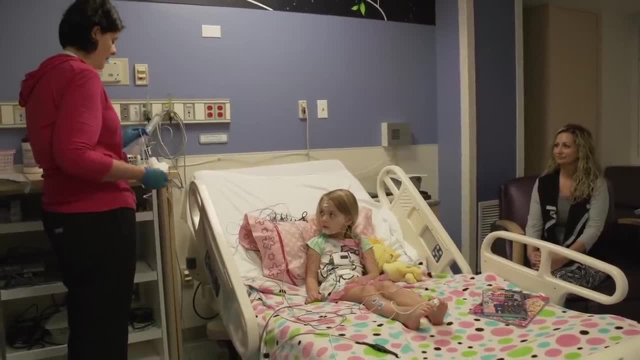 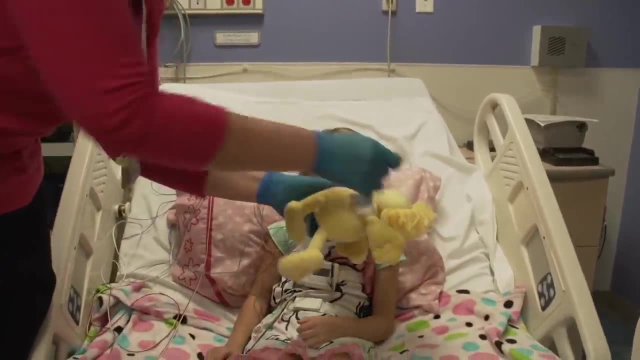 Now I'm going to put one that's going to sit right underneath your nose and on top of your upper lip, So this might tickle. It might tickle or feel funny, but it's not going to hurt. Here I'll show you what it looks like. on Woodstock. 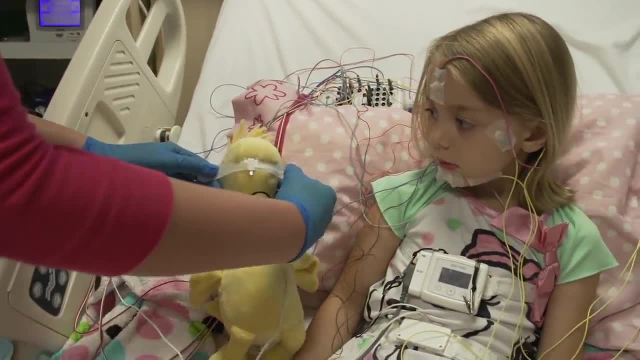 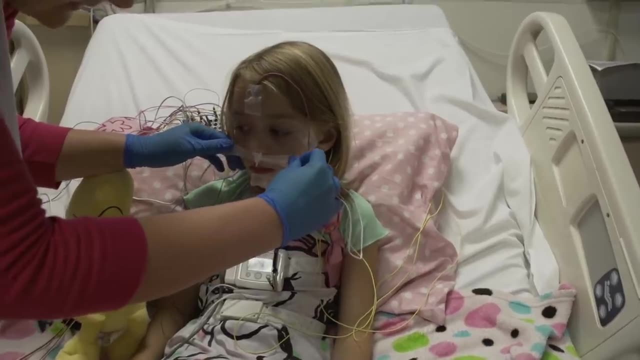 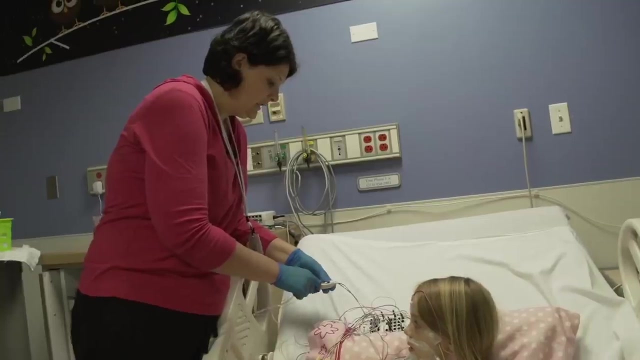 It's going to look really cool tonight. Okay, now it's Gisella's turn. Okay, you ready. Tickle, tickle, mustache. Good job. These are the most important ones tonight, because these are going to tell me about your breathing. 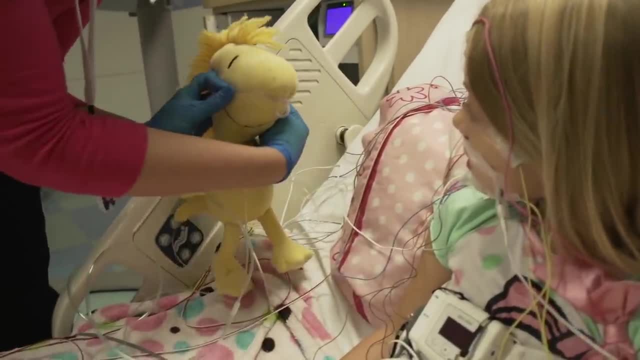 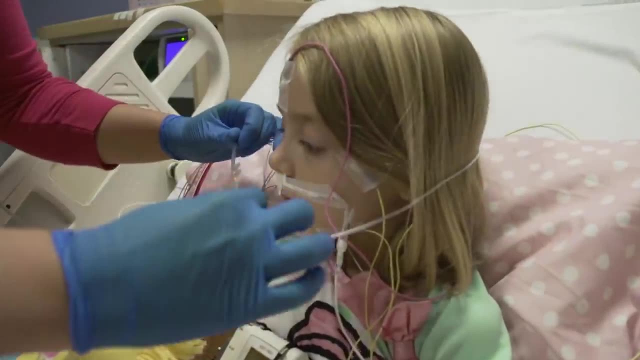 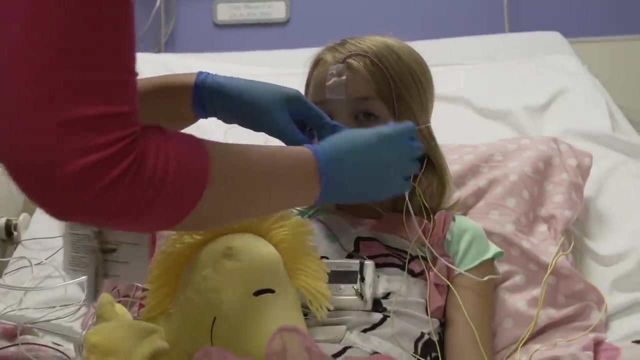 We'll show you what it looks like on Woodstock. See, Just like that, No big deal. Okay, now it's your turn. You ready, You ready, Tickle, tickle. Good job, Big girl. I'm going to put two little pieces of tape. 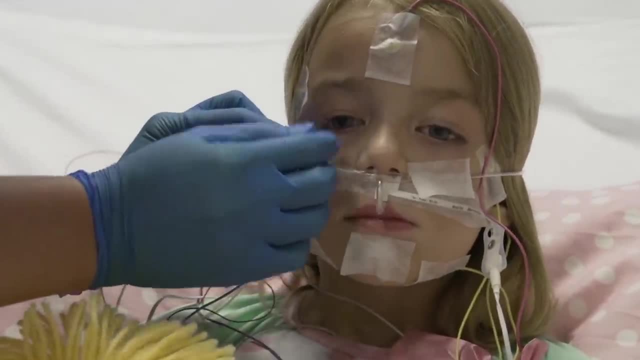 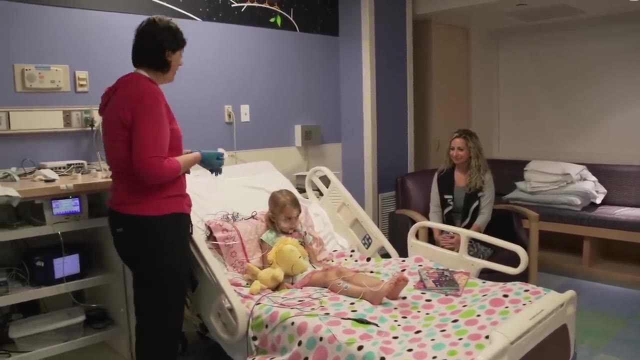 They're going to kind of hold it in your nose. Okay, Gisella, now I'm going to start putting the ones that are going to go on your head tonight. They go on with a gluey paste. It's going to leave a little bit of a residue in her hair tomorrow, Mom. 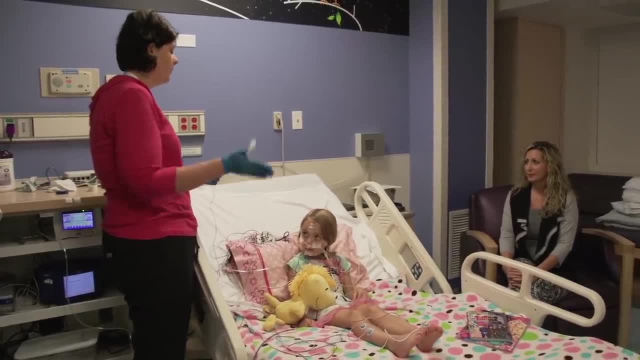 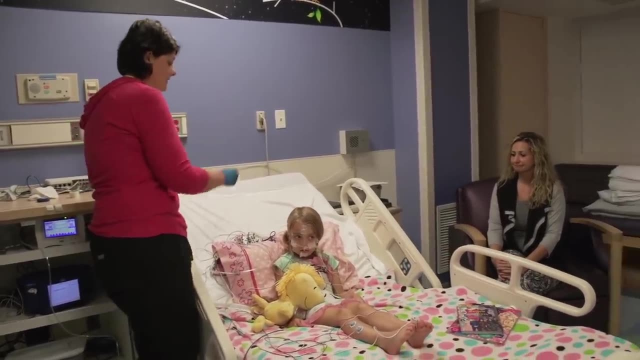 The best way to get this out is lots of warm water. Just let the water run over her head continuously for about five, ten minutes, and then it'll slide right out. okay, Okay, Okay, Gisella, to get these to stick, I'm going to push down a little bit on the top of your head.